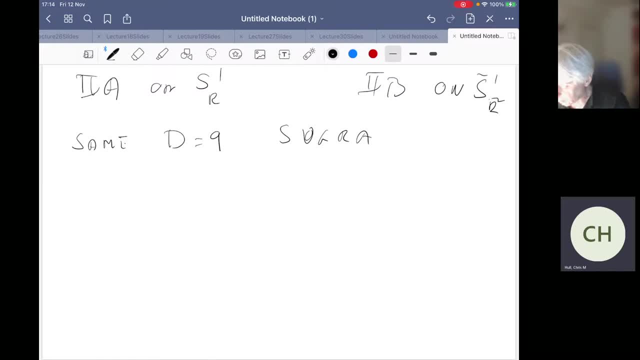 It turns out that in analysis, in the analysis of nine-dimensional supersymmetry, there are two kinds of BPS multiplet with slightly different chirality conditions which I don't want to go into in detail here, But the first one arises as the KK modes. 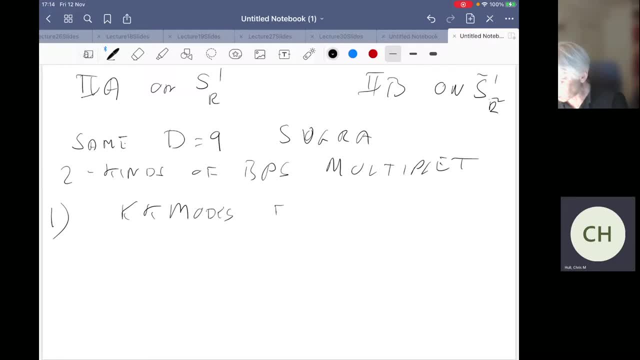 of the BPS. So the KK modes for the 2A theory on the circle or the winding modes for the 2B, And secondly the other one arises in the opposite way. So the KK modes for the 2B and the winding modes for the 2A. 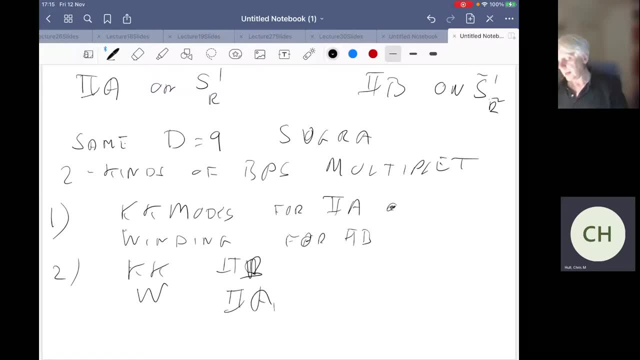 And, as we've seen before, we expect there to be a T duality which relates the theory on a circle of radius r to the theory on the circle of radius one over r. The T duality will interchange momentum and winding modes, And so this leads to the conclusion that these two must be T dual, with r tilde equals one over r. 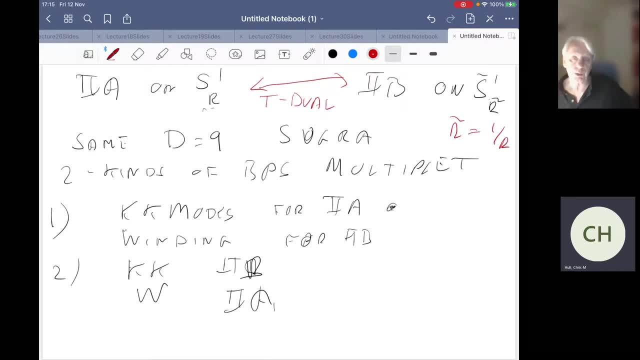 And so this leads to the conclusion that these two must be T dual, with r tilde equals one over r In units where I've set the string tension to one. So this means that the two apparently different string theories, one on a circle of radius r. 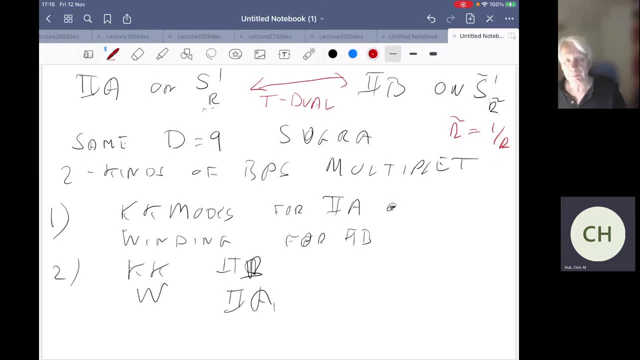 and the other on a circle of radius. one over r gives the same theory. So for when r is large, the Kaluza-Klein modes are light. The 2A theory is light. The 2A theory is light And those BPS states of the nine-dimensional theory. 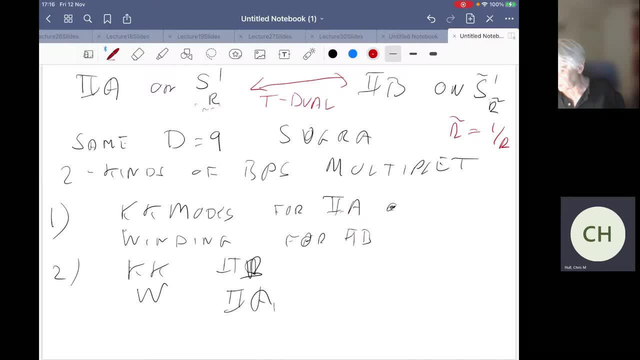 are naturally interpreted as momentum modes for the 2A theory. But as r becomes smaller, they become heavier, and then they're naturally interpreted as winding modes for the 2B string. So in this way we see a duality between these two strings. 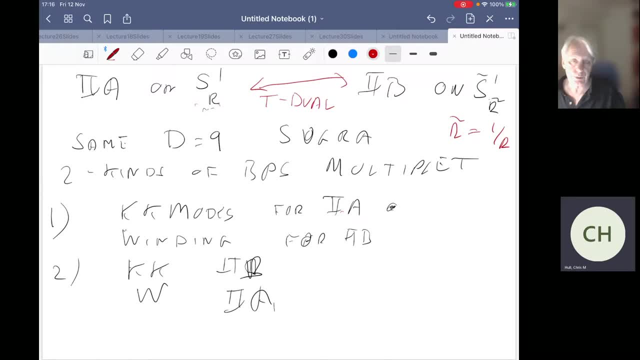 And two. we see that two apparently different perturbative string theories, when they are put on a circle, give the same theory, And in fact there's a similar story for the two different heterotic strings If you put each of them on a circle. 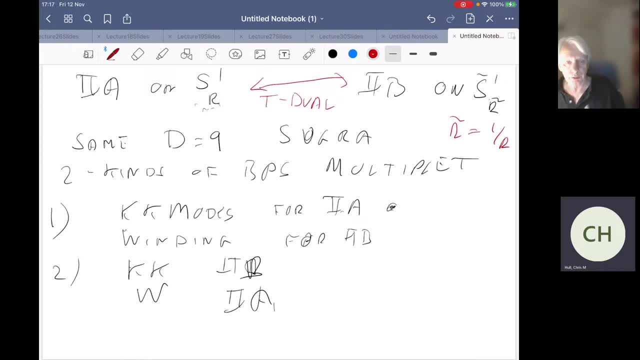 then you get the same nine-dimensional theory, And so they're part of the same moduli space and essentially part of the same theory. There's another related story which comes when we look at the SO 32, the theories with SO 32 gauge group. one is the heterotic string and the other is the type 1. 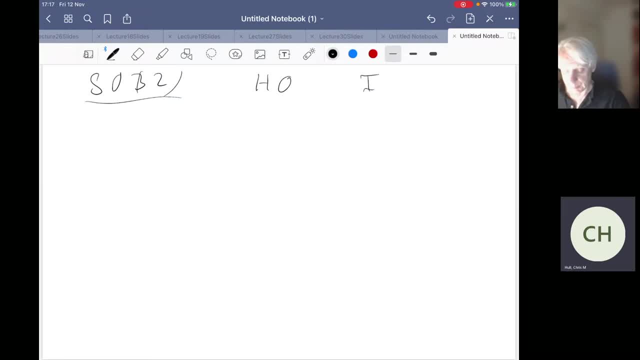 string, but each of them, naturally their perturbation theory, gives rise to different actions, or apparently different actions. but the supergravity theory, with that gauge group, supergravity plus super young mills, effective action, is unique. so they, the two, must be related by a field redefinition, and so 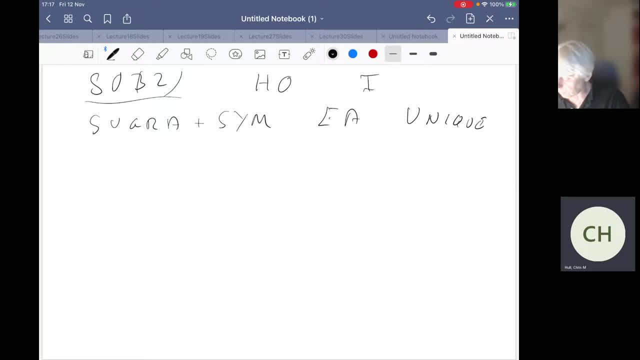 there must be equivalent theories, so they must be related by a field redefinition. and in fact the field redefinition includes a relationship between the dilaton of the heterotic theory and the dilaton of the type 1 theory in which they're related. so that means that the coupling constant of the heterotic theory is one over the coupling. 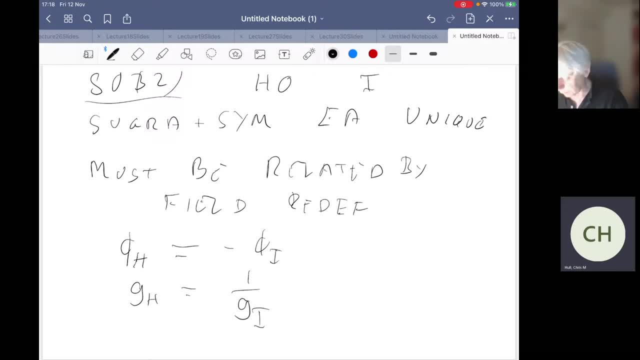 constant of the heterotic theory and the dilaton of the heterotic theory is one over the coupling of the type one theory, because the coupling constant is given by the expectation value of each of the minus two times the dilaton. and so we get that there's um a strong, weak. 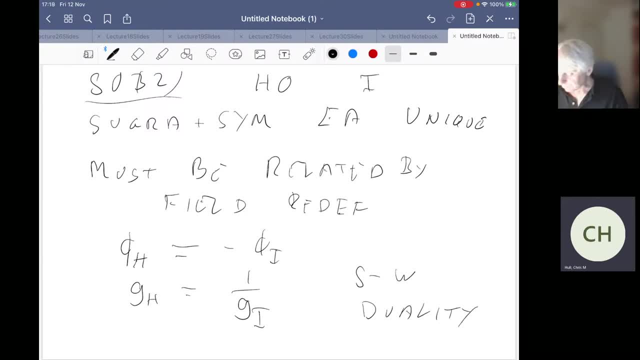 duality between these two theories and um. another story is that um that if we look at the 2a theory, compactified on a certain four-dimensional manifold known as k3, which is a compact manifold which has certain properties, uh, one way of saying what it is is that it's a four-dimensional. 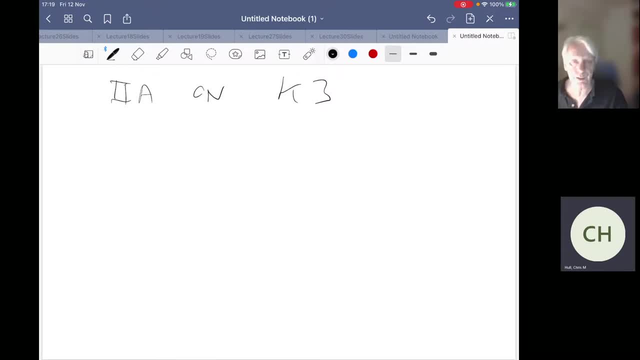 manifold whose curvature is self-dual and it's compact and it's a four-dimensional manifold. only one such manifold other than the torus which works that way. um, and if we look at this and the heterotic string compactified on t4, they um both. 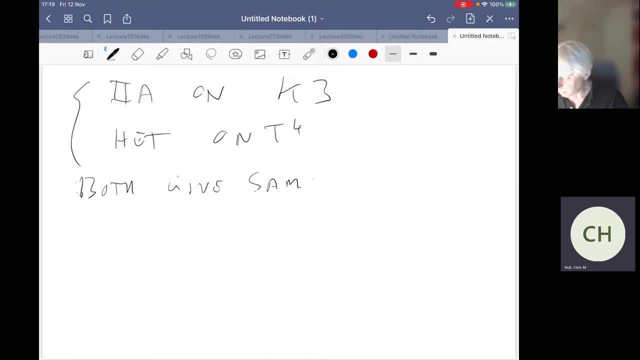 give same effective super gravity theory which has got a symmetry o for 20 cross r plus and um. in a very non-trivial check we can. you can see that one can match the bps states for the two theories and the relationship between them is another weak, strong duality. 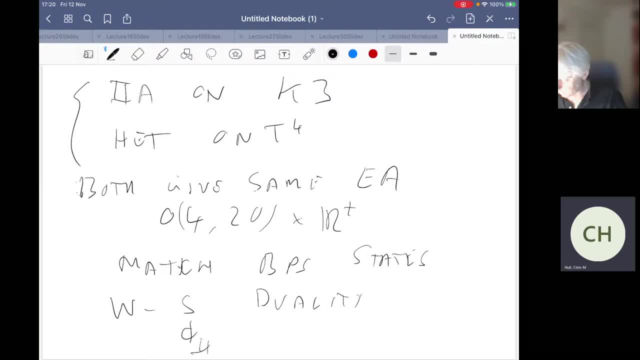 the dilaton of the 2a string. the dilaton of the 2a string is minus the dilaton of the heterotic string. um, when you uh, when you look at, uh, the effective actions which relate from all these um, the details of this and the arguments on um the previous couple of slides can all be found in the. 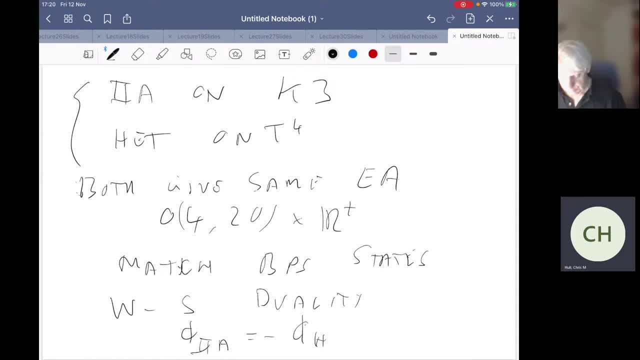 um paper by whitman and um. it's well worth reading through that um. you know this classic paper to to look at the details of these arguments. And here we see that again there's a picture that two very different string theories are giving rise, when compactified give rise to the same effective supergravity theory. 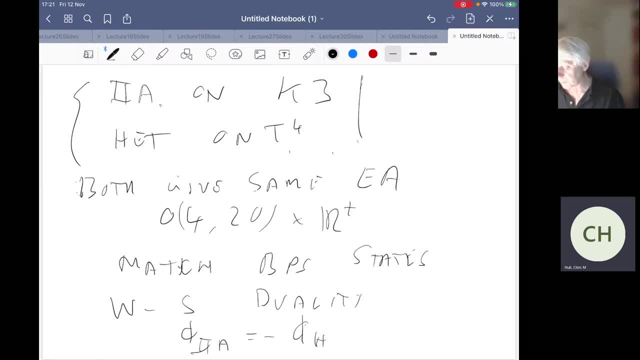 And this leads to the conjecture that they're in fact non-perturbatively dual. They're very different as perturbative theories, but the full theory is, rather remarkably, non-perturbatively equivalent. And as a final example, in some ways the most important and most dramatic one is if we look at the two: A string in 10 dimensions. 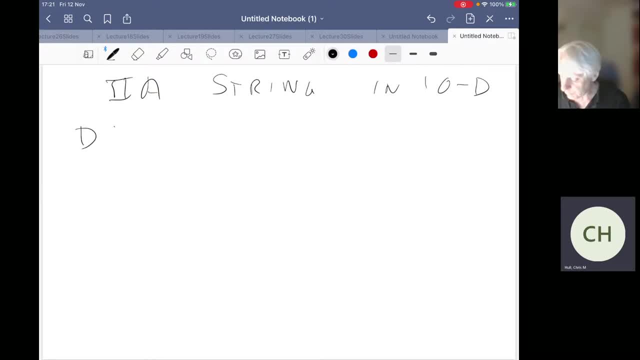 So here we've seen that there are G0 brains coupling to the Riemann-Riemann vector. So here we've seen that there are G0 brains coupling to the Riemann-Riemann vector. field Cm and their mass is given by the BPS formula and it's given by an integer divided by the string coupling constant. so n is an integer up to some factors of 2, pi and so on, which throughout this lecture I've been ignoring. 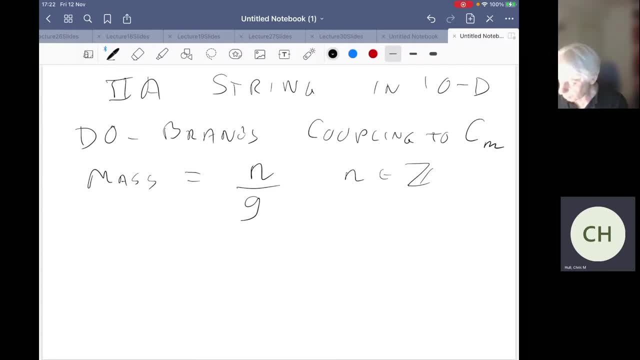 So we have. so we have n equals, so mass equals, so we have mass which is 0, well, so 0 doesn't really count. So mass: 1 over G, 2 over G, 3 over G, and so on. 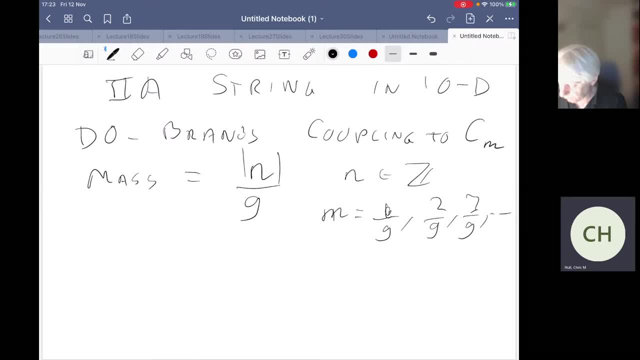 And note this is very similar to a Kulutza-Klein spectrum For a circle Of radius R, which is G. So in the limit, so as G tends to infinity, we get an infinite tower of massive modes. In the end, G becomes massless, nearly half of its ăc becoming massless. 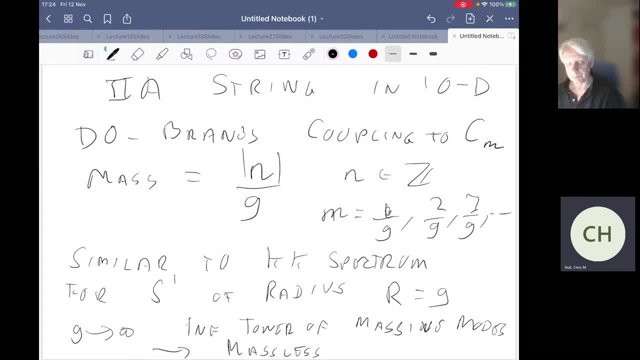 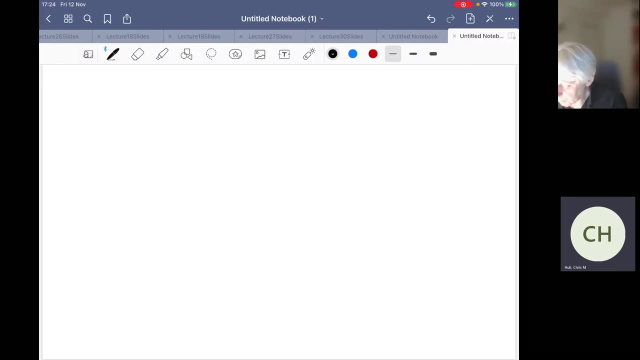 And we saw that this is exactly what we would expect in a Dekompactification limit, And this led Witten to the remarkable suggestion that the 2a string. In a decompactification limit we actually can't get an infinite tower. 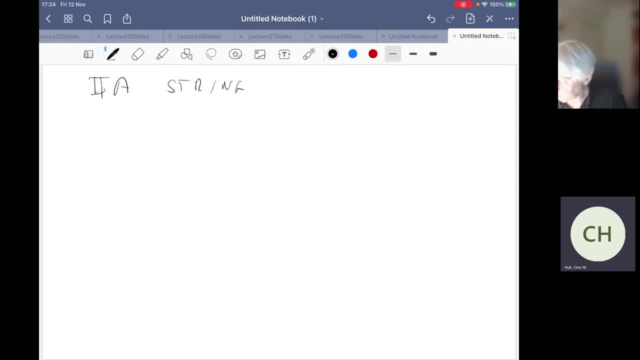 We can't get a whole K In a decompactification limit. It's unusual. It's unusual, It's unusual, It's really weird is really an 11-dimensional theory compactified on S1, where the radius of the S1 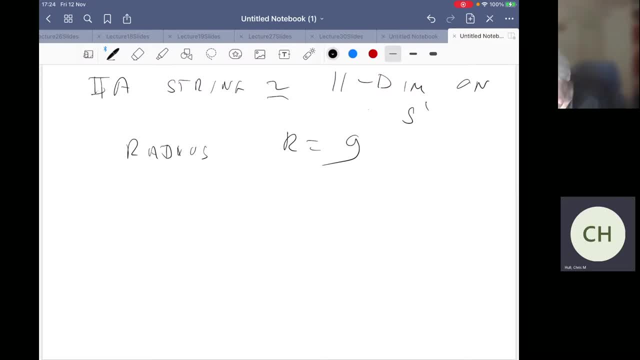 is just given by the string coupling constant, So that the limit, the strong coupling limit, is then a decompactification limit to 11 dimensions. And this is a very remarkable conjecture. but it's led to a lot of, it's passed a lot of tests. 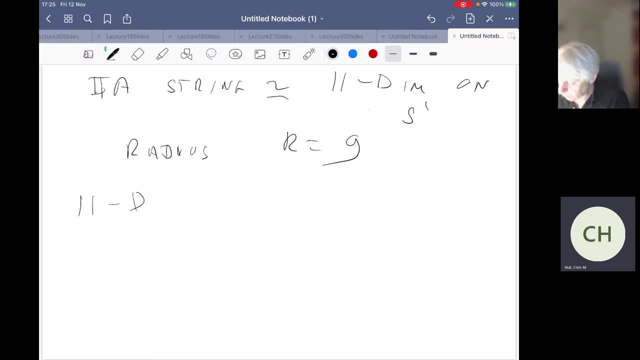 And so the suggestion: this 11-dimensional theory, this mysterious 11-dimensional theory, is one which we don't know much about directly, but it's been given the name M-theory, Maybe M for mysterious, The one thing we do know about it. 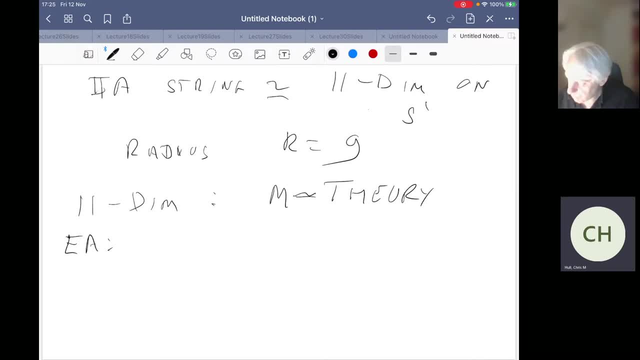 is its low-energy effective action, which is given by 11-dimensional supergravity. And this is a theory which, whose bosonic sector consists of a metric and a third-rank anti-symmetric tensor gauge field. Let's call it A-M-N-P. 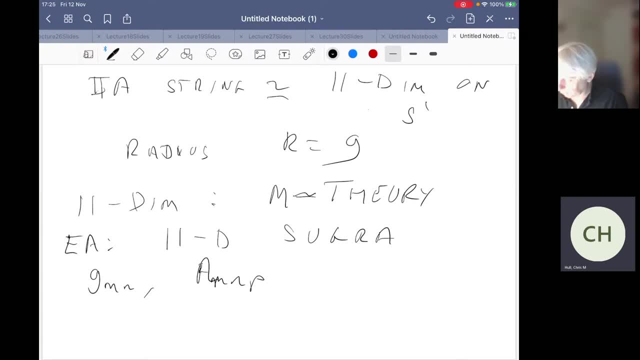 And this third-rank field will couple two membranes, which are known as M2 brains, and their magnetic duels, which are M5 brains, And when you dimensionally reduce on a circle, the A-M-N-P. Actually, let's do that on the next slide. 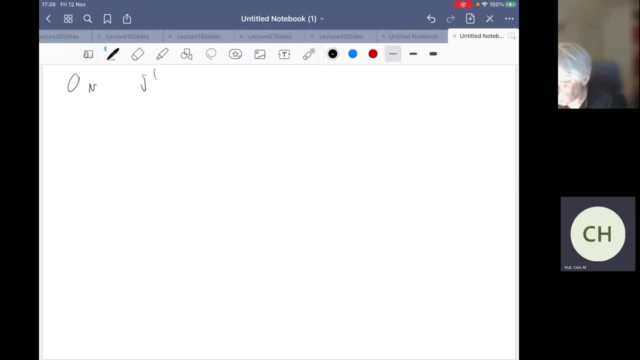 So we have the metric: G-M-N gives rise to a metric, a vector field, G-Mu-Y, where Y is the direction of the circle which is identified with the vector, with the Riemann-Riemann vector field C-Mu. 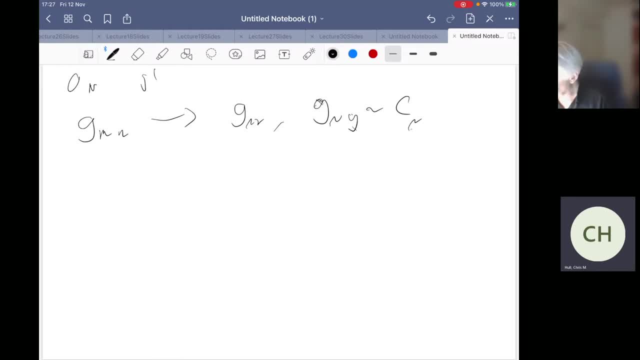 and a scalar G-Y-Y, which are identified with the dilaton and A-M-N-P, gives rise to a three-form, a third-rank anti-symmetric tensor field, which is identified with the Riemann-Riemann three-form. 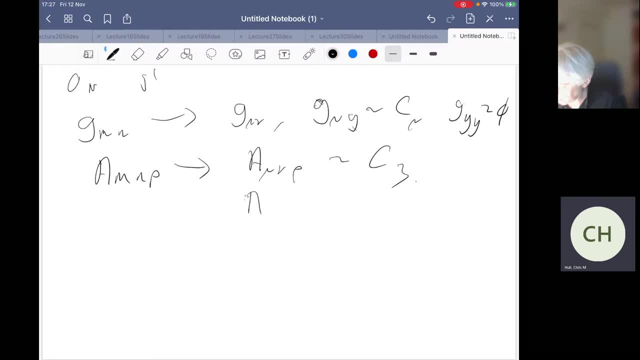 A-Mu-Nu-Y, which is identified with B-Mu-Nu, and that's all, because you can't have two Ys. It would give something non-zero. So in this way we see that we recover all of the spectrum of. 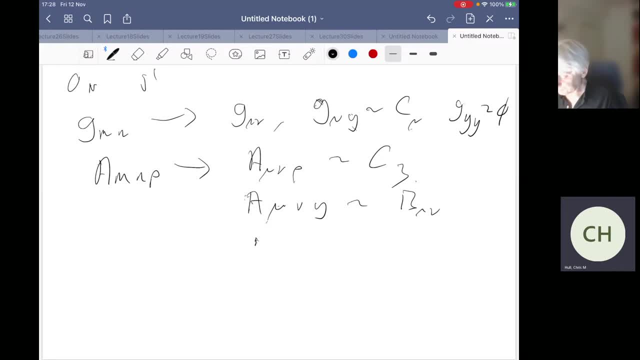 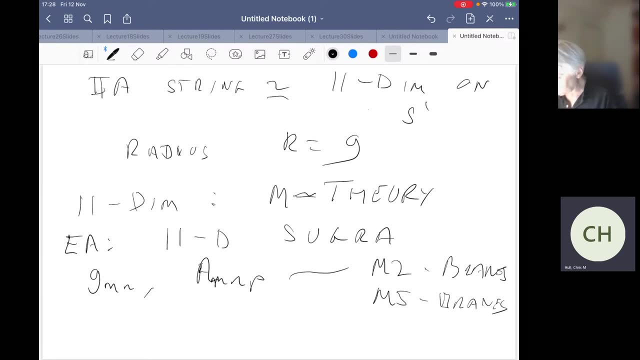 the bosonic spectrum of the 2A theory. The same work goes for the fermionic spectrum And, moreover, the wrapping the brains of the M2 theory will give rise to the brains of the sort of the M theory will give rise to the brains of the 2A theory. 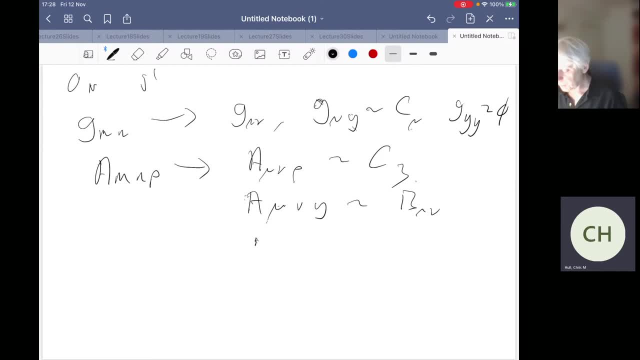 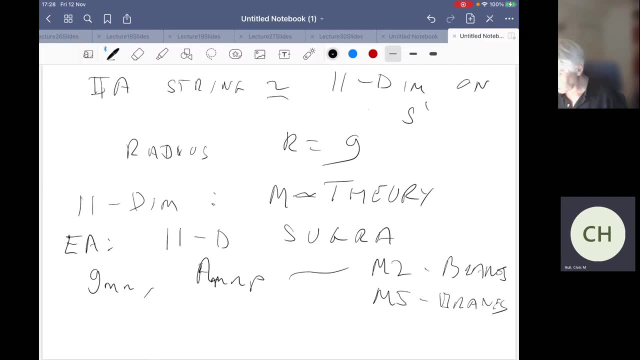 So here we see that the, in particular we see that the strong coupling limit, the dual theory, keeping the strong coupling limit of the 2A theory is rather remarkably given by M theory, an 11-dimensional theory whose low energy effective action is 11-dimensional supergravity. 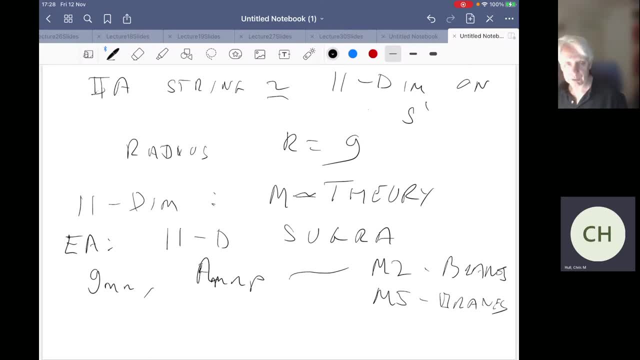 But it can't just be 11-dimensional supergravity, because it's whatever it is. it's got to give something which, when you reduce down to 10 dimensions, has got to give all the richness of the 10-dimensional string theory. 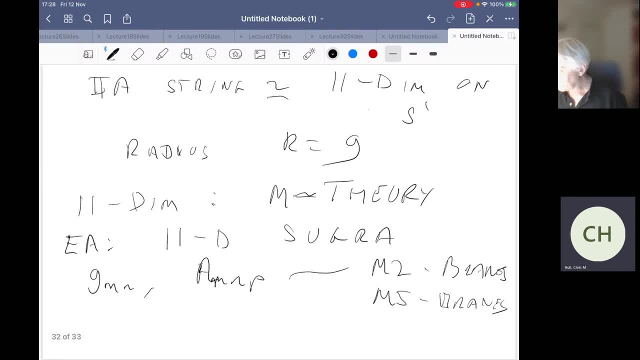 And, in particular, you've got to be able to recover all the massive string loads in principle from that story. So, to conclude, we've started off with five different string theories: The 2A, the 2B, the heterotic. 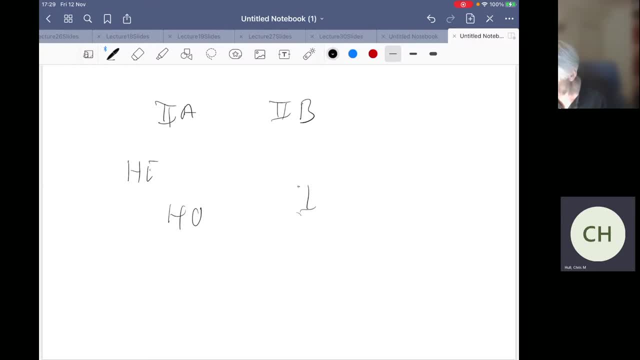 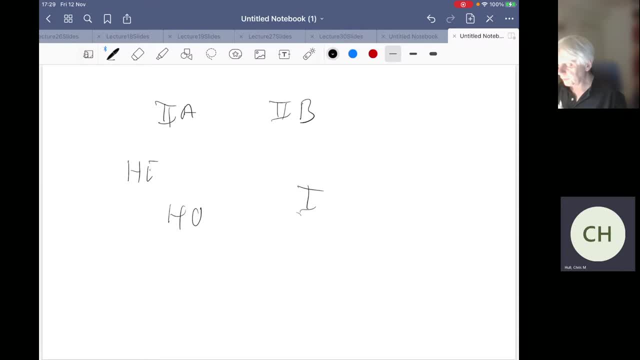 and the Type 1 theory, and what we've seen is that there are links between all of them. We've seen that there's a T duality relating a 2A with a 2B theory. There is a putting, In other words, putting the 2A on a circle. 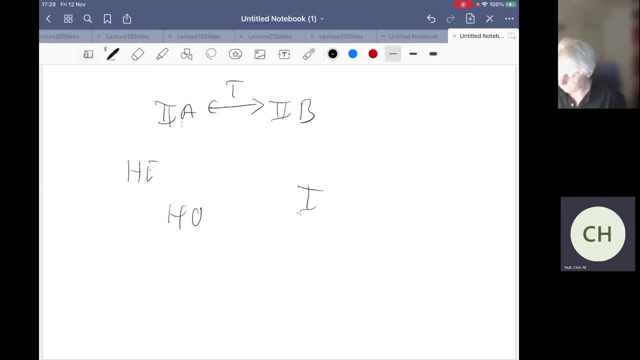 and that gives the same theory as the 2B on a circle. Similarly, putting the two heterotic string theories on a circle, they give rise to the same theory, so that once so there's a circle, there's no distinction between those theories. we've seen there's a strong, weak coupling duality between the um well, i mentioned 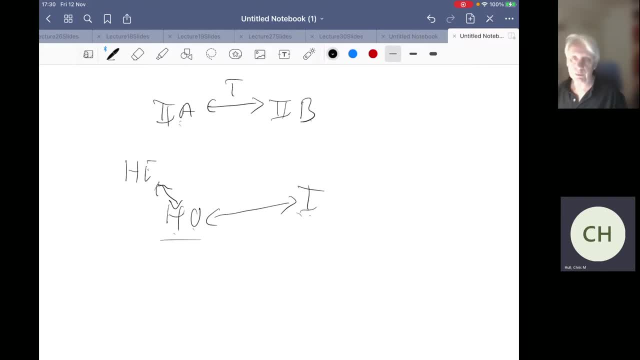 briefly, there's a strong weak coupling duality between the type one and the so and the so32 heterotic theory. which means that if you take the type one theory to this theory um of um open strings and closed strings and look at a strong coupling limit, it turns out the strong coupling. 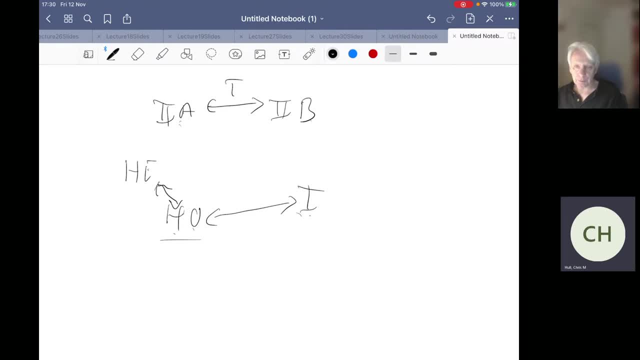 limit is. um could be described as a perturbation theory in one over the uh. in the inverse coupling of the type one theory and this perturbative theory, um is in itself a string theory, but it's a very different string theory from the one that we started with. it's given by the heterotic string. 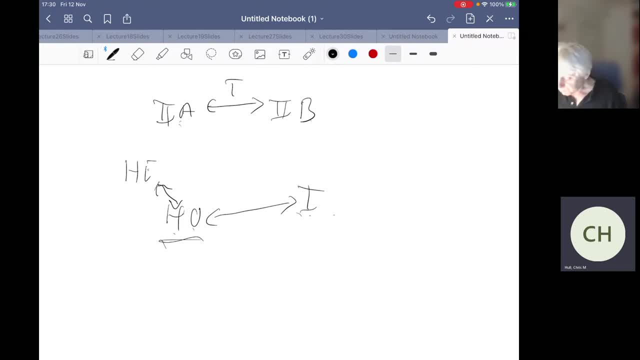 theory and, conversely, um, this, um. i didn't have time to talk about this, but the strong coupling limit of the 2b theory is again the 2b theory. uh, but the um the 2b theory, but it's, it is. they're related by an? s part of the sl2z symmetry: u duality symmetry. 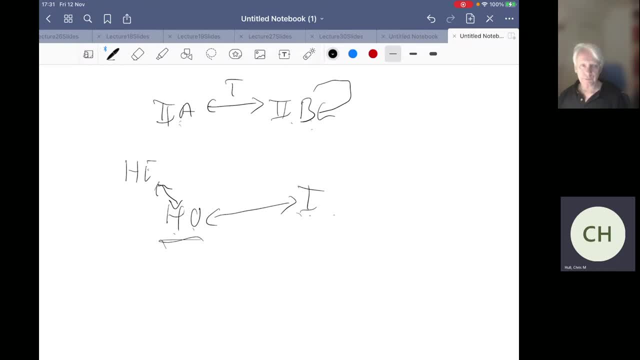 which arises here um. but whereas in the four dimensions the sl2 interchanged um the electric and magnetic charges, in the case of the 2b theory it interchanges the charges carried by the fundamental string strings, or the nervous Schwartz, never Schwartz strings, and those carried by the um, the d strings. 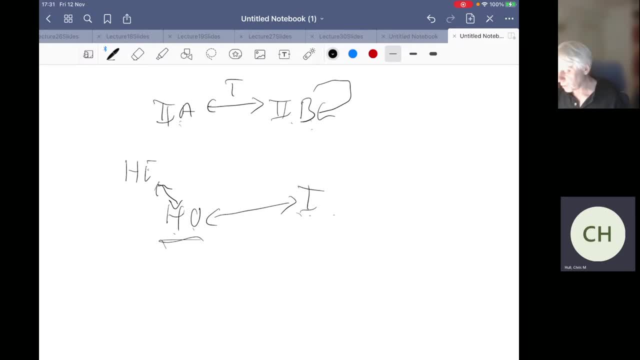 and um. it interchanges those in in that way and um. moreover, we've seen that- this I've also mentioned briefly- there's a strong, weak coupling duality here between 2a on k3 and the heterotic string compactified on t4. so the 2a 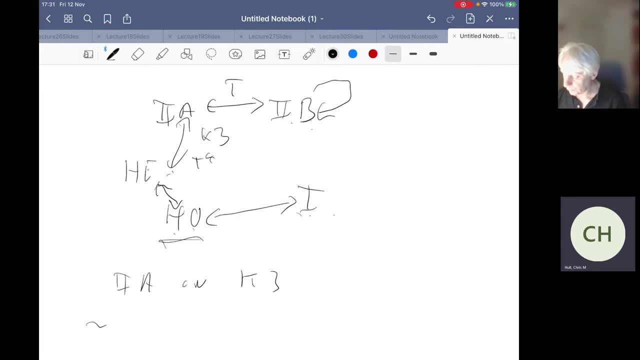 on k3 is the same as the 2b as as the um, the heterotic string on t4. so this is quite dramatic. these are very different looking string theories and the fact that they turn out to be non-perturbatively the same. it's very strange. 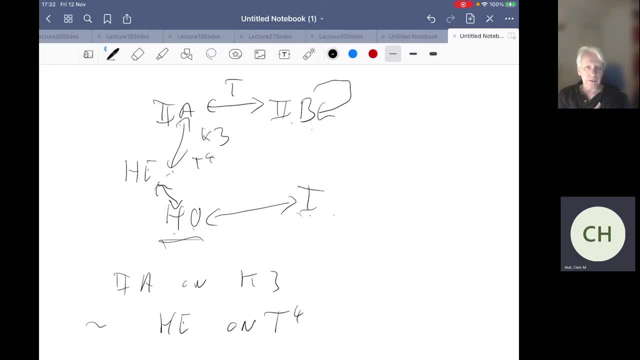 and striking in particular um our prejudices and intuition that are based on the low energy effective field theory gives um a lot of importance to the space time manifold in which you're um acting, but here we're seeing that this, that um the same string Theory, um would interpret the geometry in two different ways. in the 2a picture, um you'd interpret 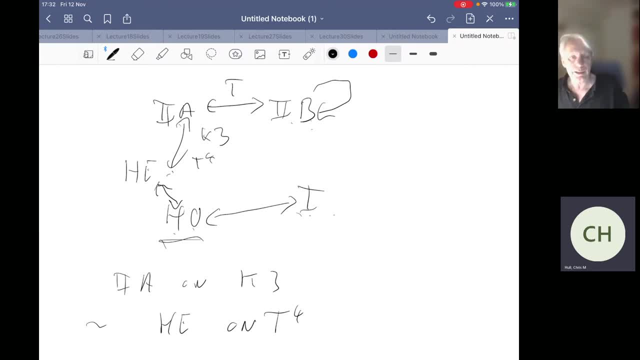 the internal geometry as being k3 and in the um heterotic picture, um, you'd interpret the internal being T4.. In the sense in which both are right, just as in general relativity, when you're looking at the physics, if you look in two different coordinate systems you describe. 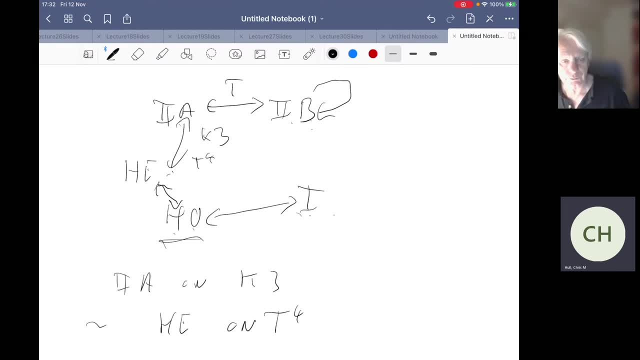 the same physics. Here there's a in this generalized sense, because you've got the diffeomorphisms enlarged to or enhanced to these extra stringy symmetries. These extra stringy symmetries go beyond those of general relativity And in this context it means 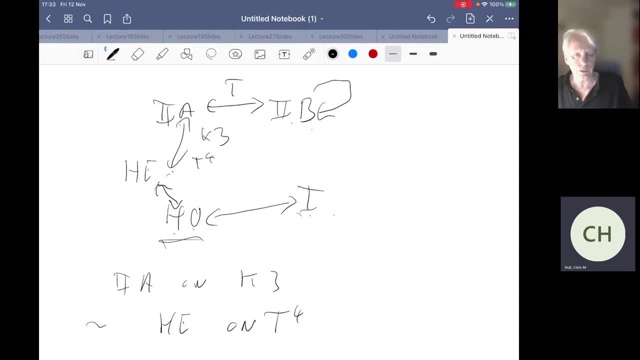 that the K3, what looks like K3 when the theory is viewed as a 2A theory, is seen as a T4, a four torus when we look from the point of view of the heterotic analysis of the same theory. And, moreover, there's a strong coupling limit of the 2A theory which gives 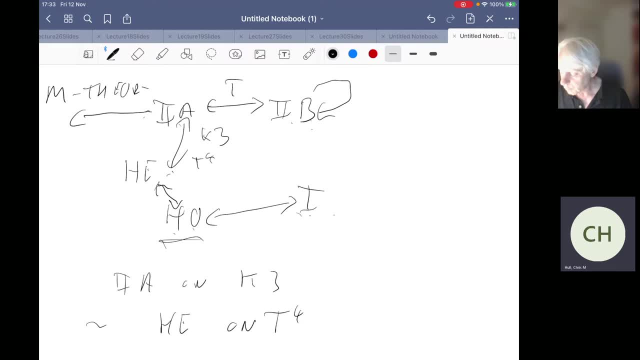 rise to M theory. There's an 11-dimensional limit where, which is M theory and M theory on a circle of radius R is equivalent to the 2A string theory as a coupling constant, G. So when the radius is small it looks like a weakly coupled string theory in 10 dimensions. But as you increase, 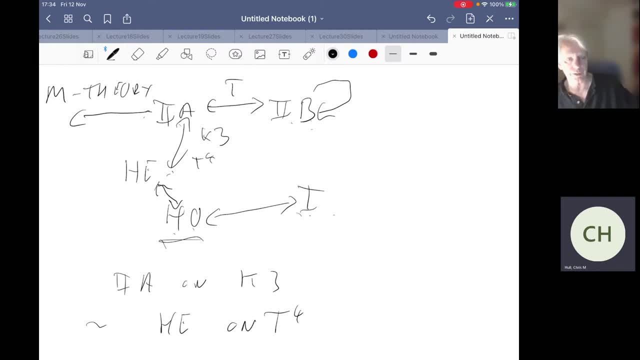 the 2A coupling constant, or that corresponds to increasing the radius of the M theory circle and it looks more and more like an 11th dimension. So if you start off with the perturbative theory, which is the 2A given by the 2A super, 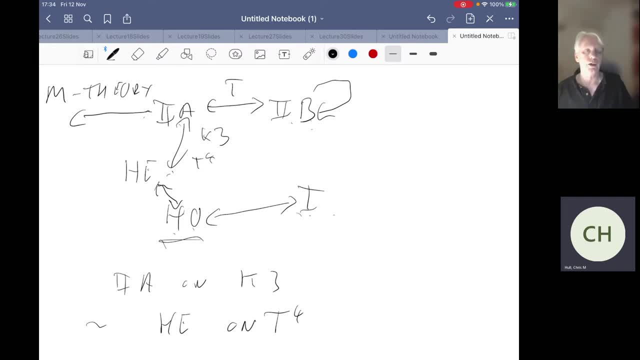 string perturbation theory and extrapolate that to strong coupling. what you find is that as the coupling gets larger, the theory no longer looks like a 10-dimensional theory but becomes like an 11-dimensional theory, And one finds that 11 dimensions emerge in. 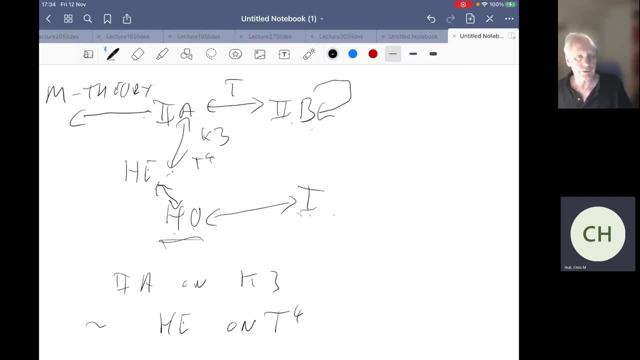 the strong coupling limit, And one finds real evidence that the strong coupling limit is a 10-dimensional limit. And one finds that 11 dimensions emerge in the strong coupling limit, And one finds real evidence for that, that, for example, there's really 11-dimensional Durant symmetry emerging. 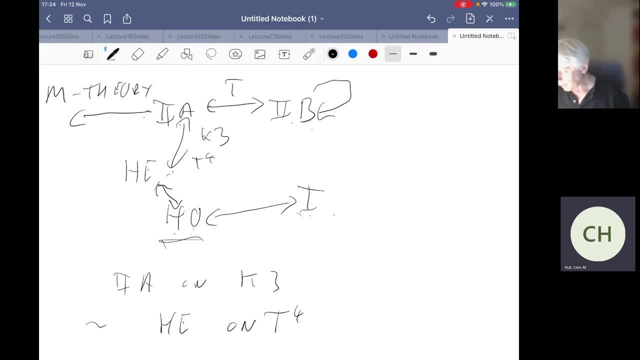 and it really is an 11-dimensional theory. But in this way we're seeing that we've found arrows joining up all of the different string theories. So, following these arrows, we can take any of the five different string theories and then link it to the others. 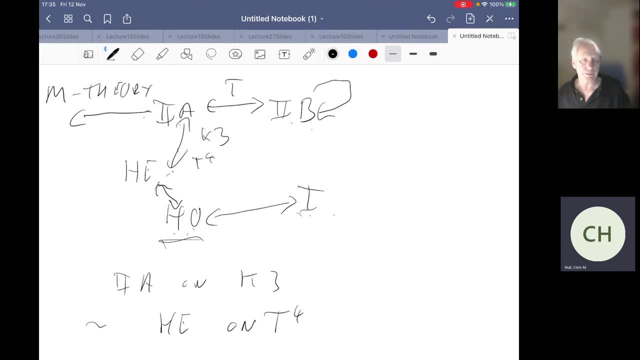 So that means that whereas as perturbative theories there are five distinct theories, they're all essentially seen as different parts of the same theory. They're all linked together. So there's this big theory which contains all of them, And M-theory is seen. 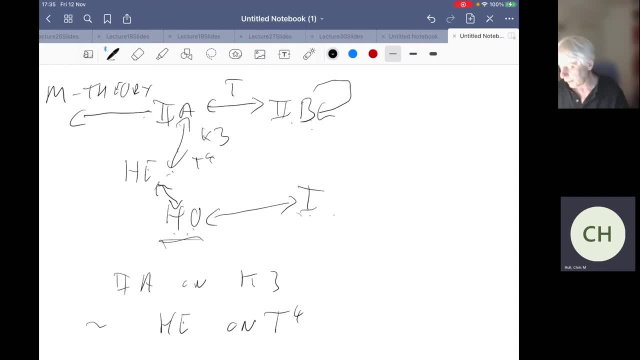 as the theory which gives rise to all of these different theories And, in fact, starting from the 11-dimensional M-theory, there are constructions which give rise to each of these different theories, albeit going via putting that on a, putting the theory which is the. 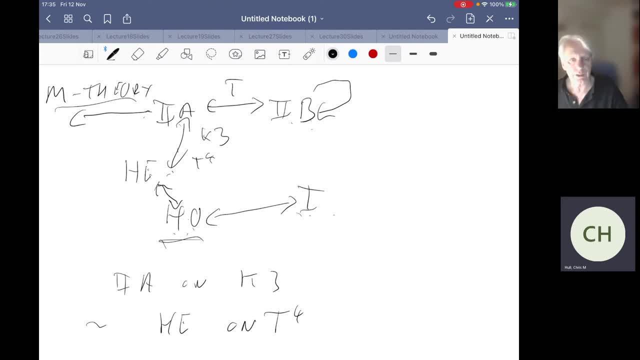 theory on a torus or on K3 and going through a chain of interactions. So in this way we see that, instead of there being that, we're seeing all of the different string theories unified in one theory. So the question about why are there five different quantum gravity? 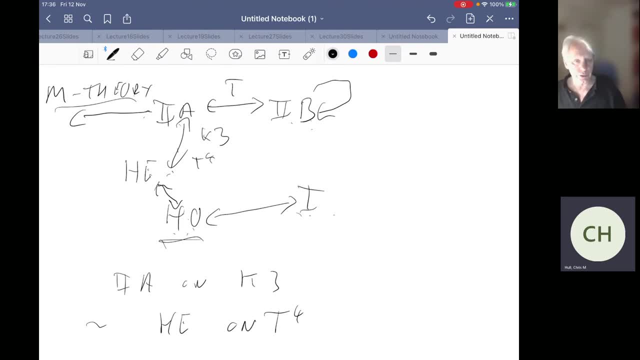 theories have a dramatic answer in fact saying no, there are not. When you look at these non-perturbatively, they're all different facets of the same theory. And When I was giving a lecture on this soon after the Witten's paper in 1995, I found a nice 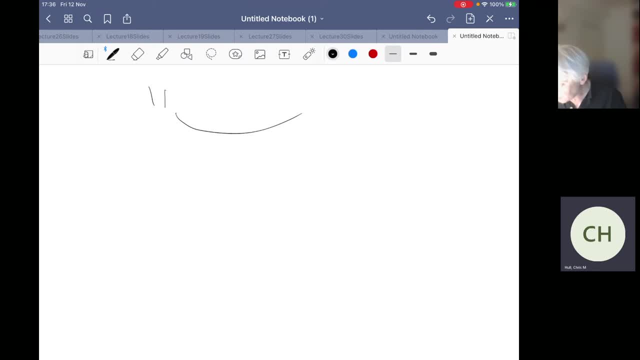 diagram which I thought suggested a nice picture encompassing all of these, this structure. So we have some picture of the moduli space, So we're thinking of a moduli space, and then going off in different, different limits will give rise to different, different aspects of the theory. 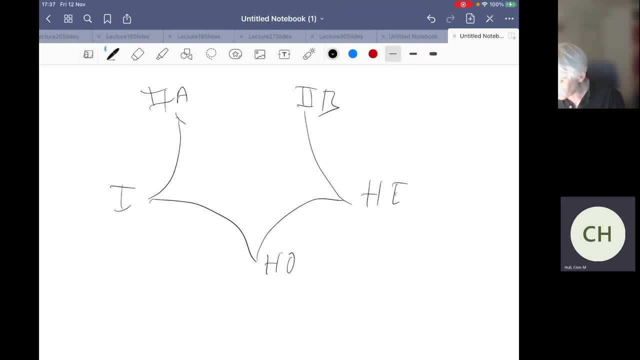 So perhaps I'll have one more cost giving 11-dimensional theory. And so these could be thought of as all different. Each of these different perturbations, Theoretical theories, could be thought of as different corners, different limits of this underlying theory which we we still have very little control or understanding of. 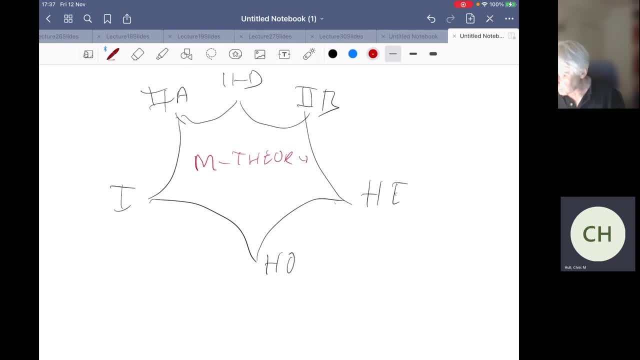 But it's been given the name M theory and we can think of different. we can we understand it in different corners of the moduli space, where a particular one of the particular moduli is such that it becomes a small coupling constant. in one corner, The theory could be analyzed as a perturbative to a string and another as a perturbative to the string and another. 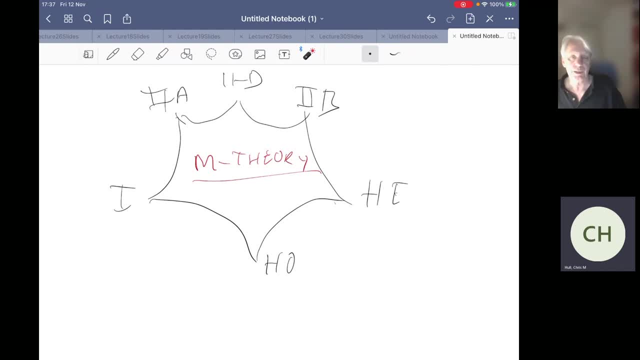 It's a theory which looks whose low energy limit is 11 dimensions, 11 dimensional supergravity, and and so on. And so we have this rather satisfying picture where we have all of these different, apparently different- string theories arising as different corners of one underlying